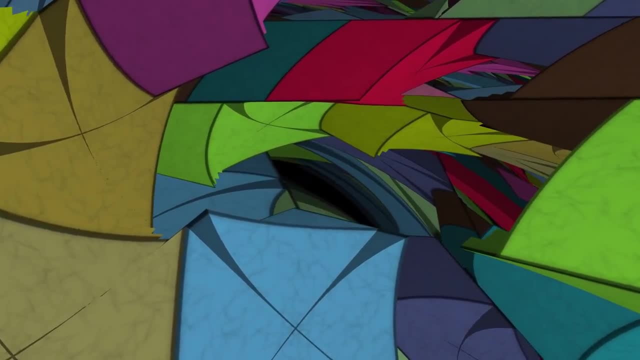 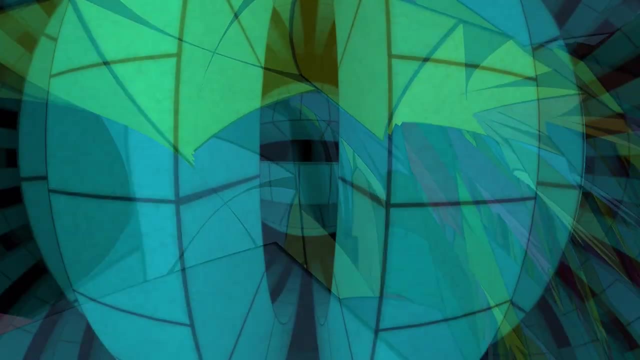 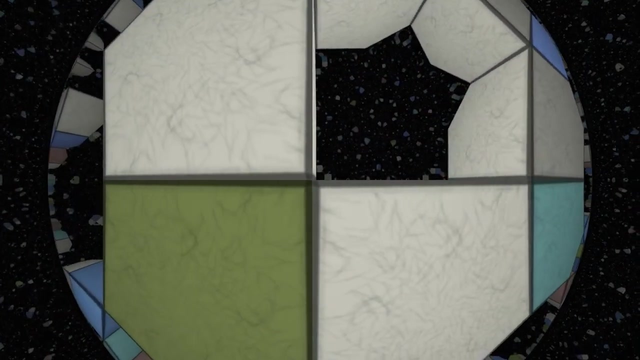 Hello, Many of you have asked us about nil geometry. In this video we will try to explain how this geometry works. Let us recall that there are some shapes that are impossible in the Euclidean geometry. However, they are possible in the non-Euclidean geometries, For example, right-angled. 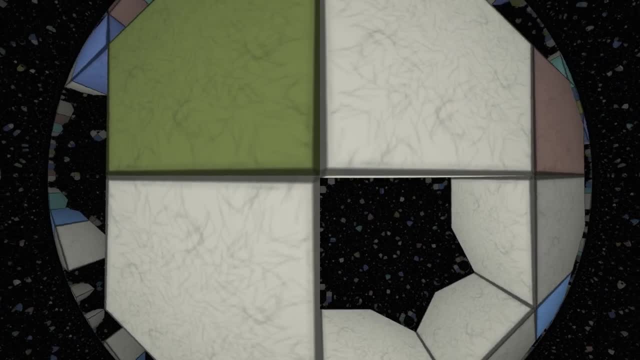 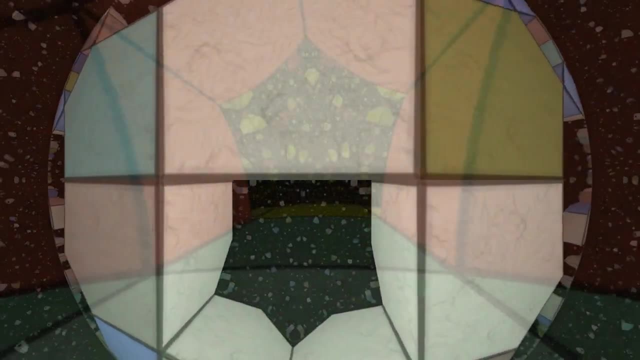 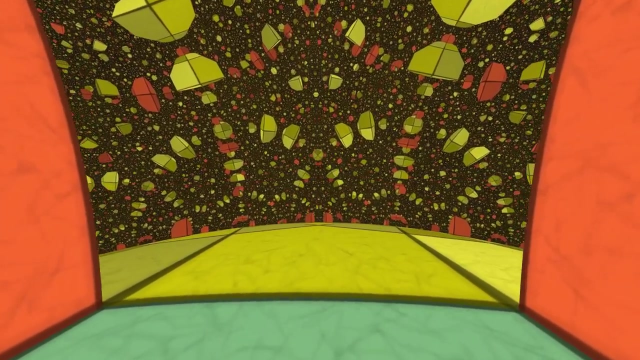 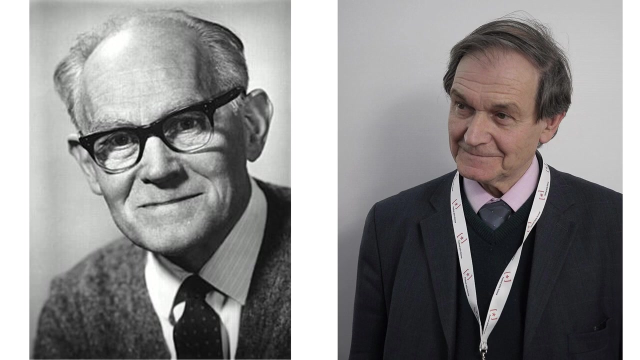 pentagons are possible in hyperbolic geometry. If you haven't seen such exotic shapes yet, we recommend our other videos. See the link in the description. However, today we will deal with a different kind of impossibility. In 1959, Leonel Penrose and Roger Penrose had constructed an impossible figure called 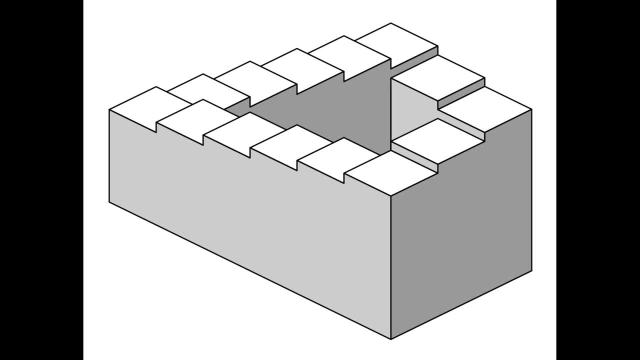 the Penrose staircase. At the first glance, the staircase looks like a projection of a valid Euclidean construction, But it is true that the staircase is not Farewell from our view. So why is Penrose staircase? Well, I will show you the vídeos using Euclidean algorithms. In this video, I will try to explain for you why in Europe. 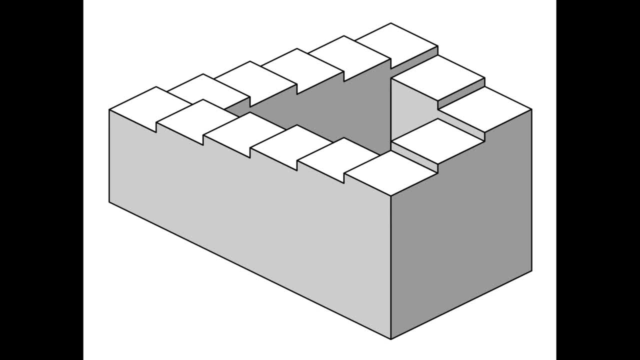 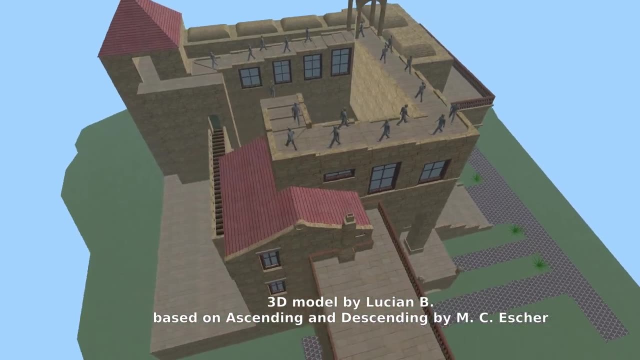 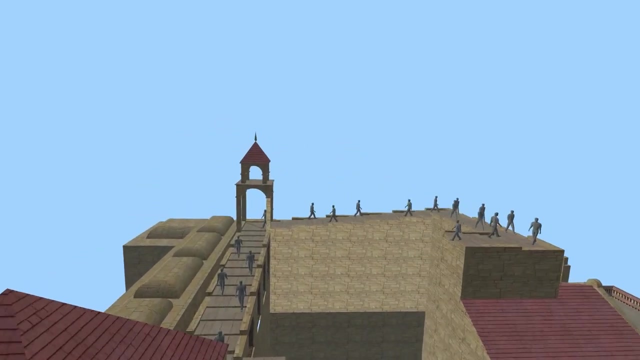 But a closer examination reveals that it is not spatially possible. It seems we could not construct a three-dimensional model of such a staircase, Or could we? No, this was just a perspective trip, But why are we talking about those impossible figures? 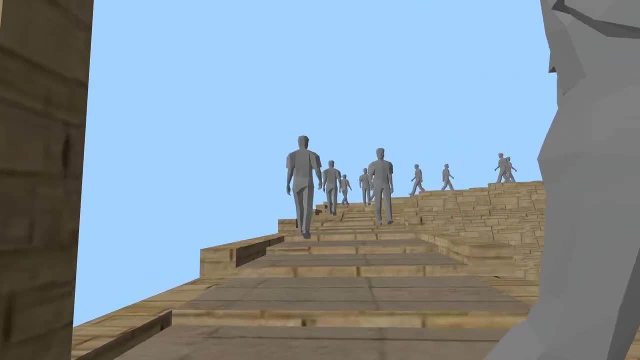 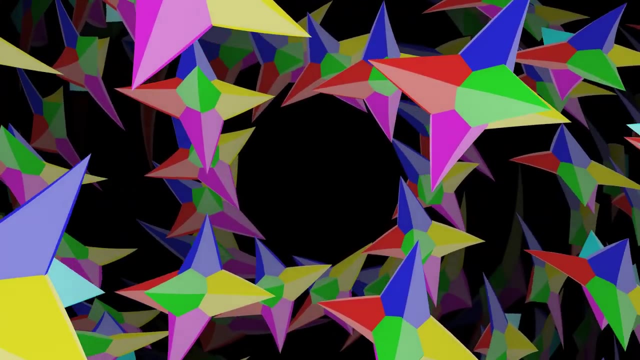 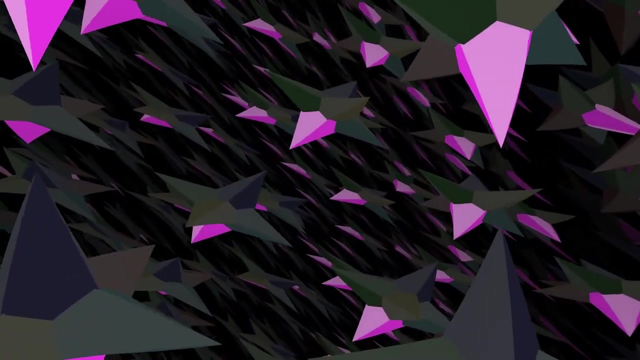 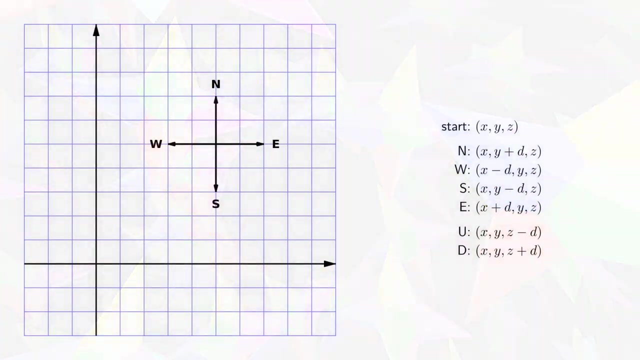 Do they have some relation to nil? Let's find out. Nil is a three-dimensional geometry. Every point has three coordinates. We can move in six directions, which we will call north, east, south west, up and down. In the Euclidean geometry. moving in one of these directions by one unit simply changes. 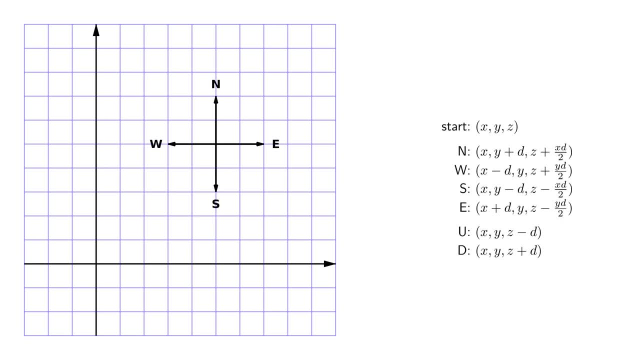 the matching coordinate by one. In nil it is a bit more complex. Moving north, east, south or west also changes our z coordinate, Euclideanいたま. Let us imagine a tool in the Euclidean geometry using directions north, east, south and west. 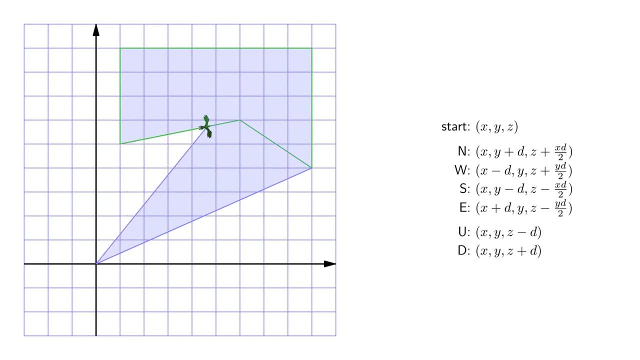 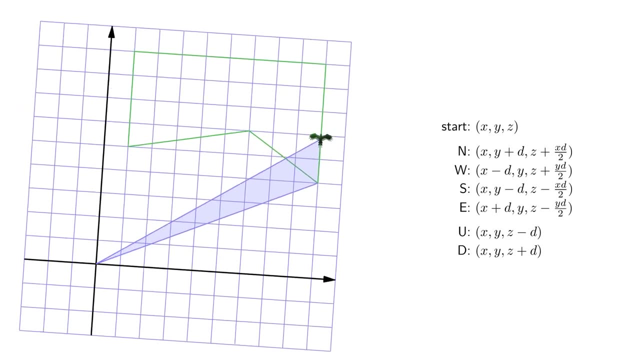 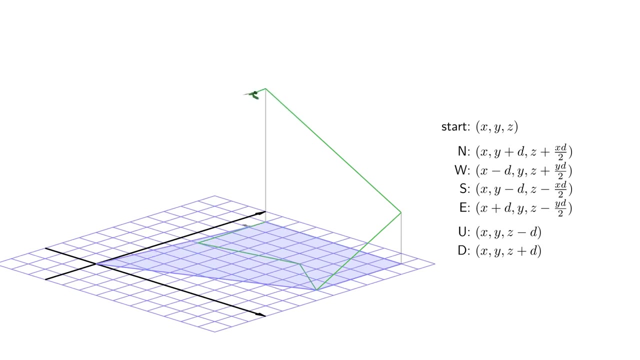 such that we return to the starting point. It would be a kind of loop. If we recreated the same steps in near geometry. we would end up directly above or below the starting point, with the difference in the z-coordinate proportional to the area of the. 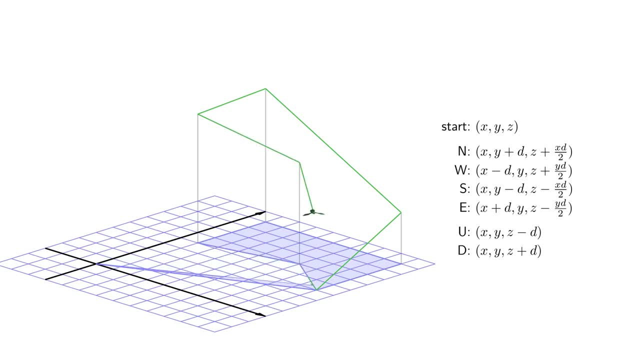 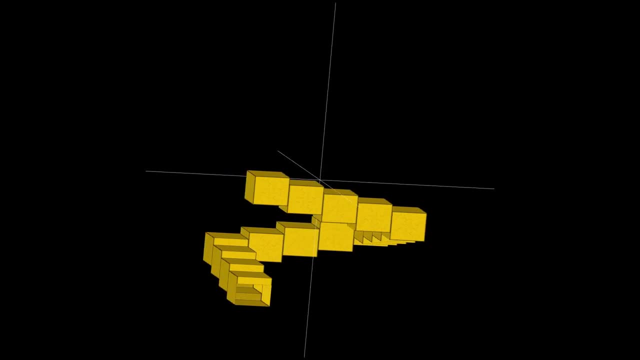 loop. So let's use this behavior to recreate the Penrose staircase. First, let's try to use this behavior in the Euclidean geometry. We build every step lower and of course, after one loop we end up lower than we started. 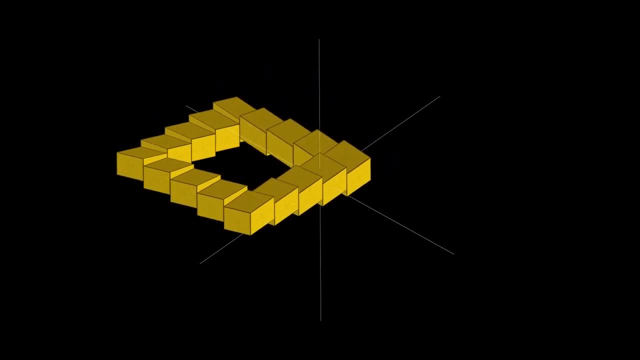 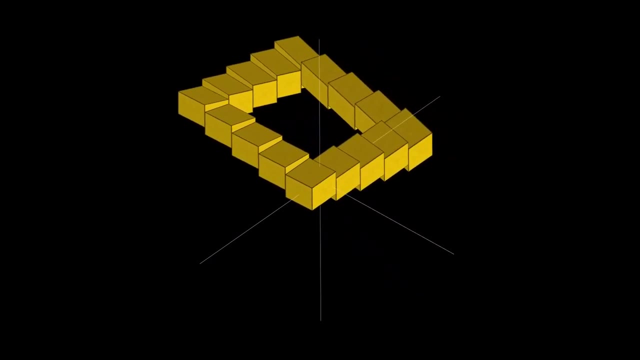 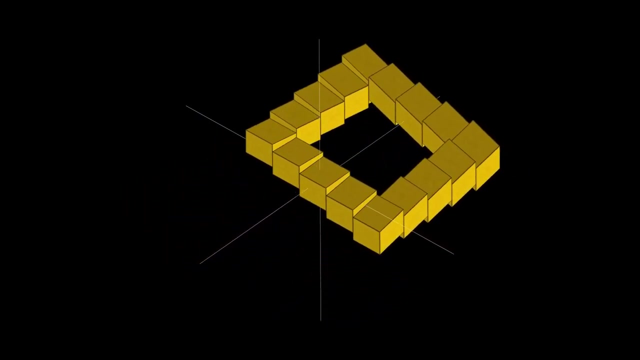 so the staircase does not cycle. Now let's use the magic of nil to recompensate the lost height. We can create the staircase that we can descend forever. This animation may look a bit like cheating, but this is because we are showing a Euclidean. 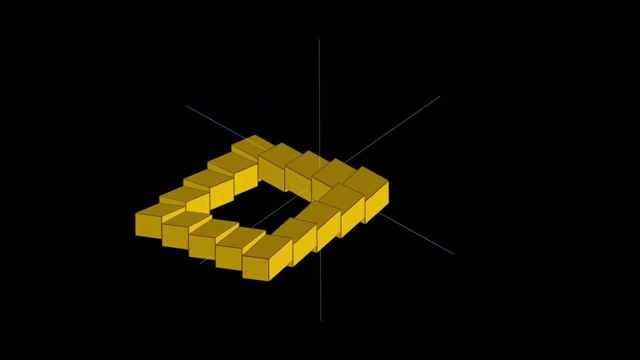 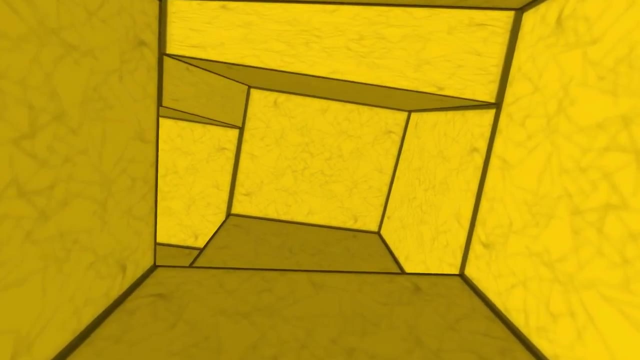 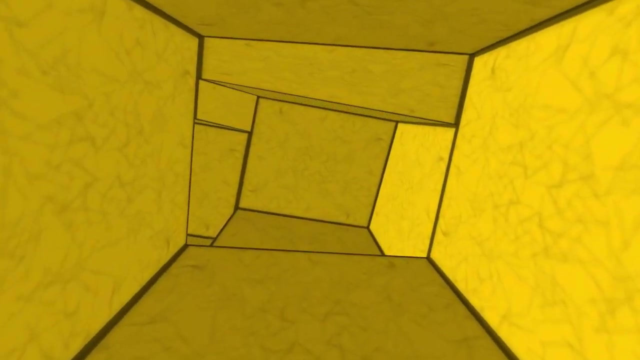 model of nil. It is not what the inhabitants of such strange world would see, So let's become those inhabitants. Here are our stairs. in the first-person perspective. from the inside, You might notice an unexpected effect: that the world seems to spin. Why does this happen? 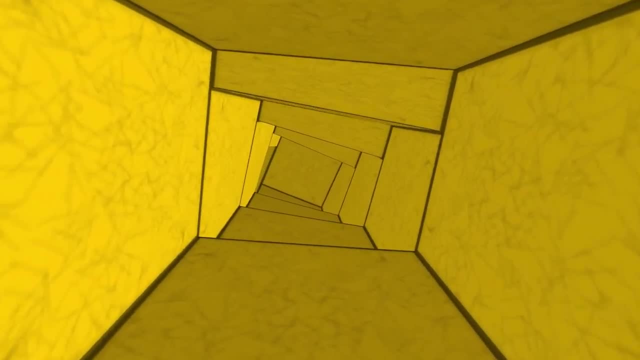 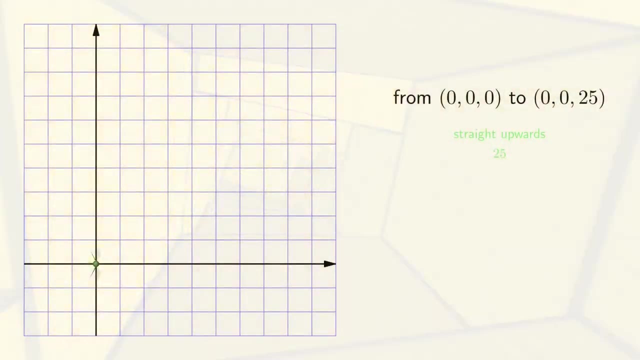 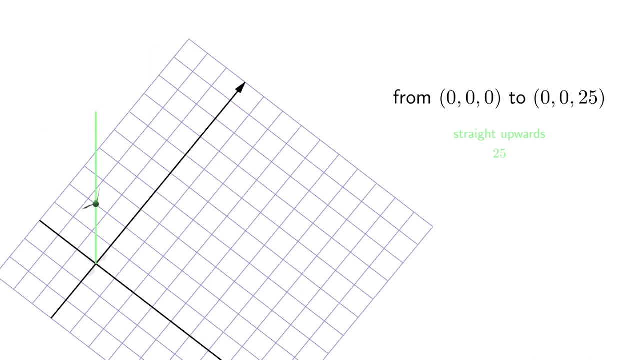 Why does this happen? According to Fermat's principle, the path taken by a light ray is always the shortest one. To understand how light works in nil, let's think a bit about moving from 0, 0 and 0 to 0, 0 and 25.. 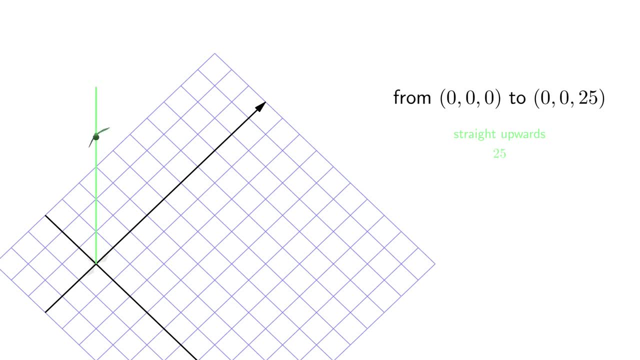 First, there is an obvious path of length 25.. But can we do it better? Yes, we can. Here is a square of edge length 5.. Since such a square has an area of 25 and a perimeter of 20, it takes us to 0,, 0 and. 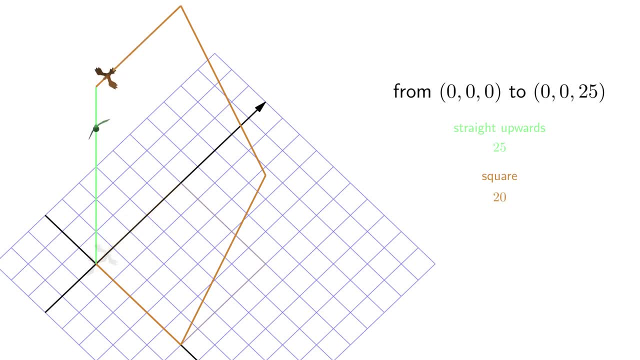 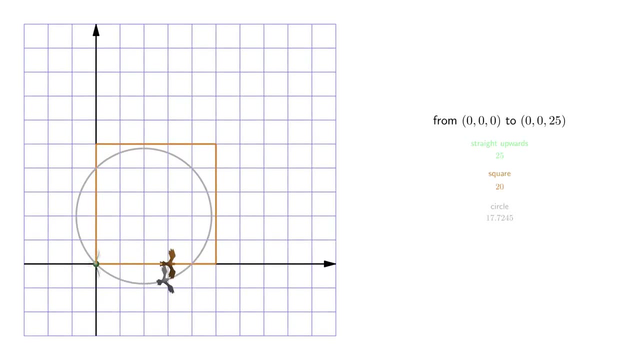 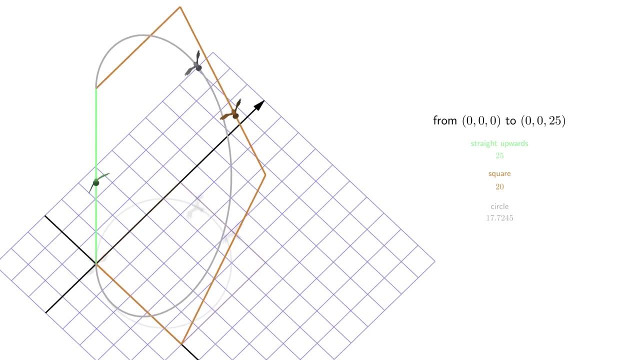 25 in just 20 steps. We can do even better. Quindado has already known that among shapes with a given area, the circle has the shortest perimeter. Moving a circle with an area of 25 will give us a shorter path that will lead us quicker. 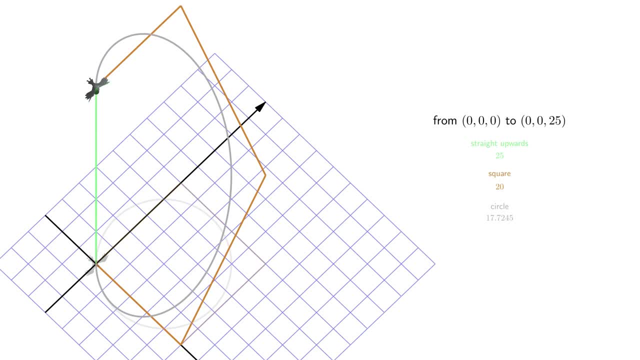 to our destination. But that is just the silver medal. For the gold medal we need to combine the silver and the green paths. We make the circle slightly smaller and we satisfy the difference by moving slightly upwards. The length of such a path can be computed using the Pythagorean theorem and minimized. 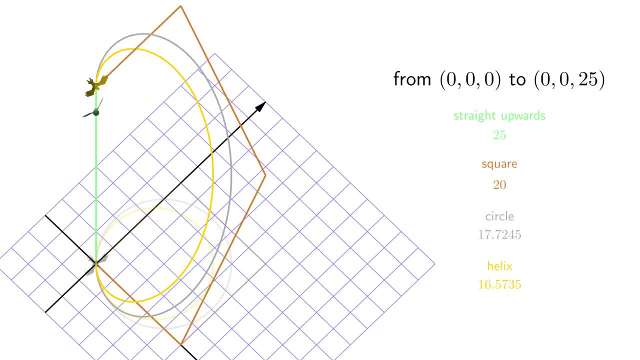 The length of such a path can be computed using the Pythagorean theorem and minimized by moving slightly upwards. The length of such a path can be computed using the Pythagorean theorem and minimized by moving slightly upwards. The length of such a path can be computed using the Pythagorean theorem and minimized. 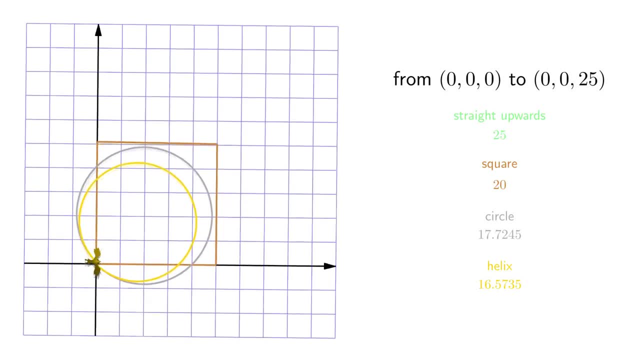 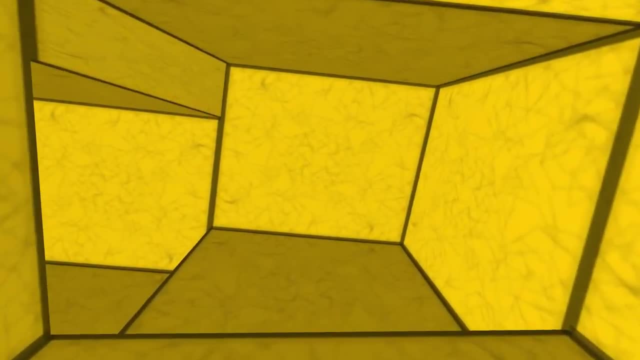 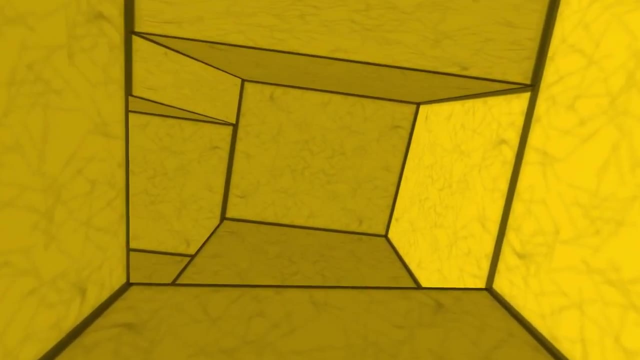 by moving slightly upwards. But that is just the silver medal. There is the optimal radius which yields the best path In Neel. the light-ray paths, called geodesics, are like the ones we have just constructed. They are helices – the steeper the helix, the smaller its radius. 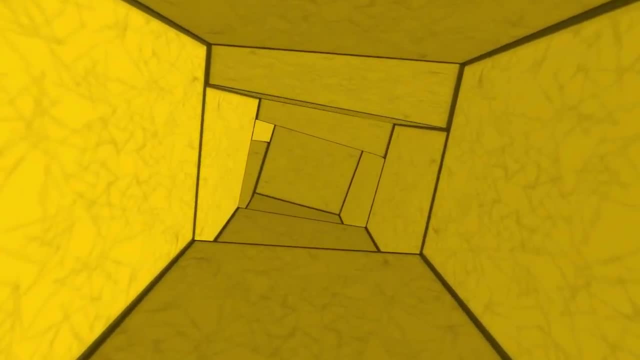 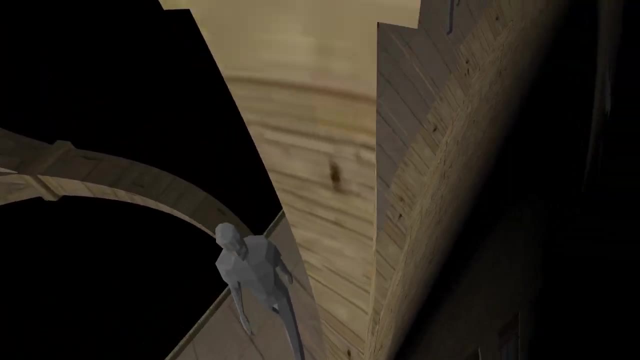 The view appears to spin because of this curved shape. The person is moving slightly upwards. If you are curious about these shapes, go to the link in the description of the video. impossible figures work in Nil. see the description for our other videos. 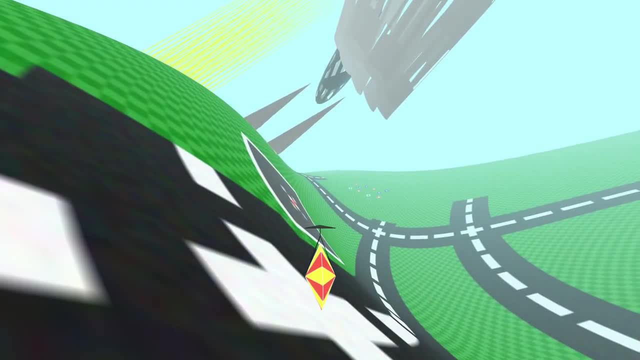 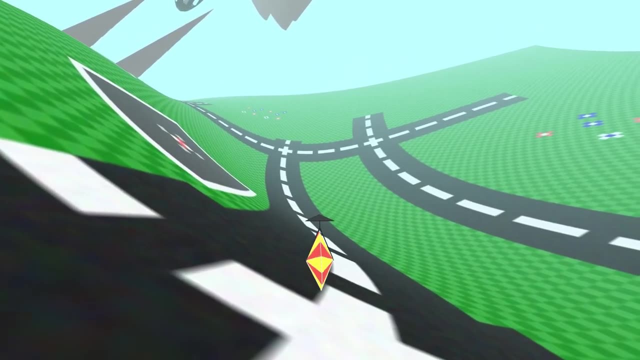 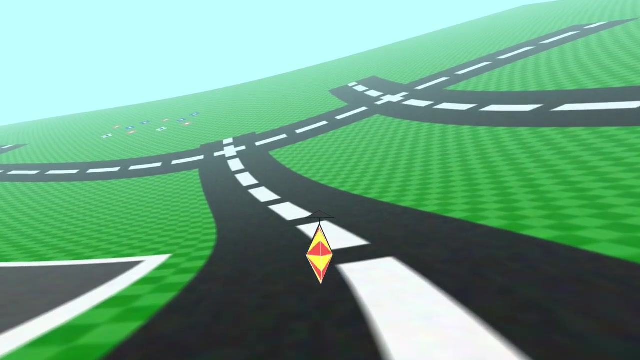 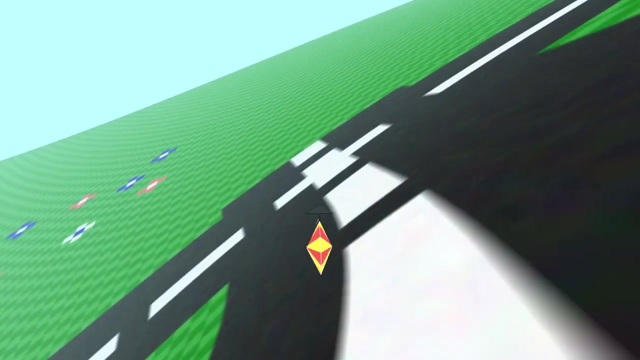 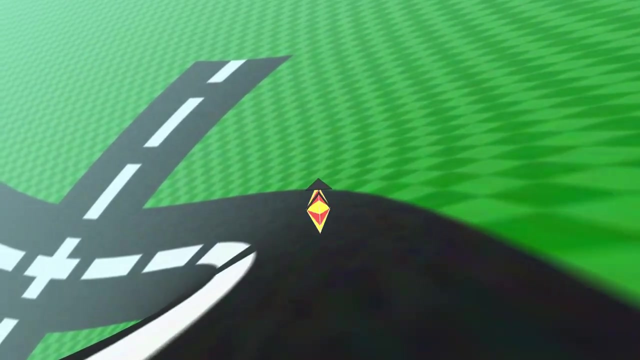 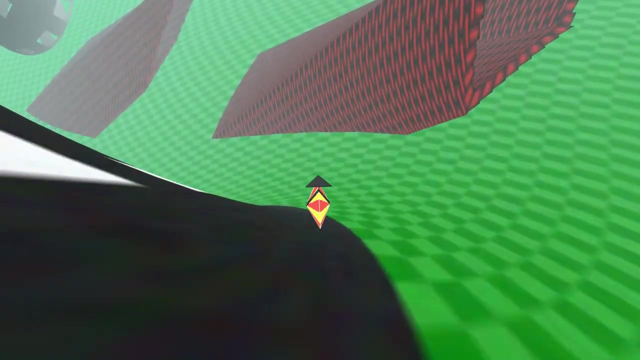 And as the last treat here is a landscape in Nil. The unicycle here is using the magic of Nil to go faster and faster. Look how the landscape appears to shift as we move. Thanks for watching and have a nice day. Have a great rest of your day. Have a great day. Have a great day.